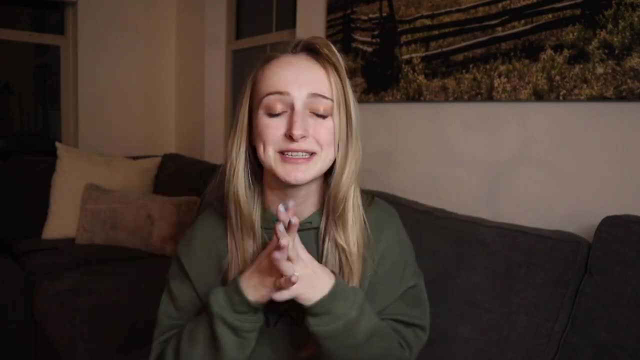 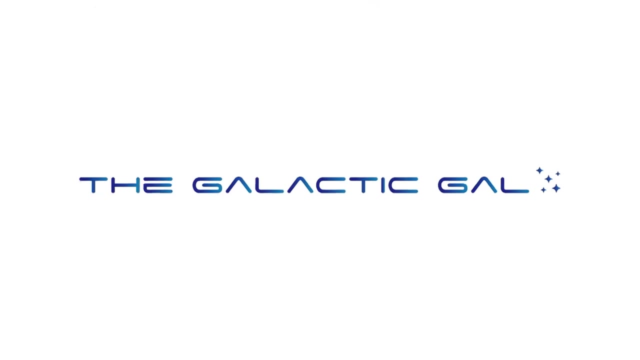 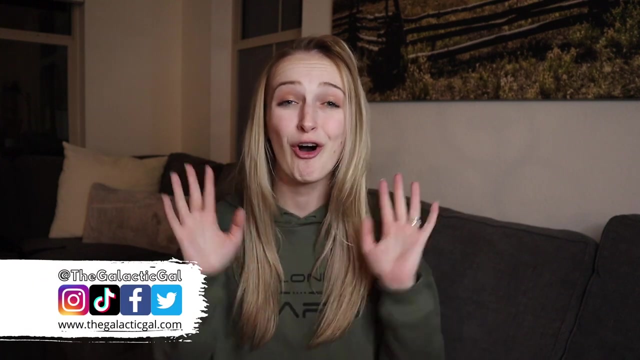 Have you ever looked up into the sky and just wish that you could sail amongst the clouds or the stars? Well, I have the perfect job for you. Hi everyone, welcome back to my channel. My name is Camille the Galactic Gal, and today we are going to be talking all about. 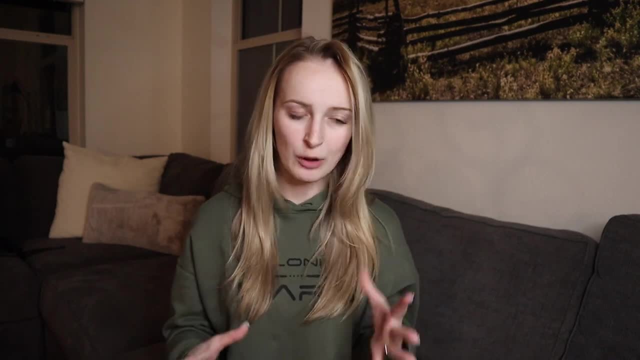 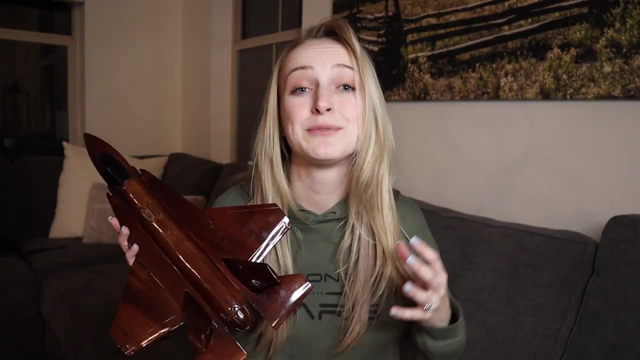 aerospace engineering. So what is aerospace engineering Like? what does the word actually mean? The word aerospace is a combination of aeronautics and astronautics. Aeronautics comes from the Greek words for air and sailor. Astronautics comes from the Greek words for space and sailors. 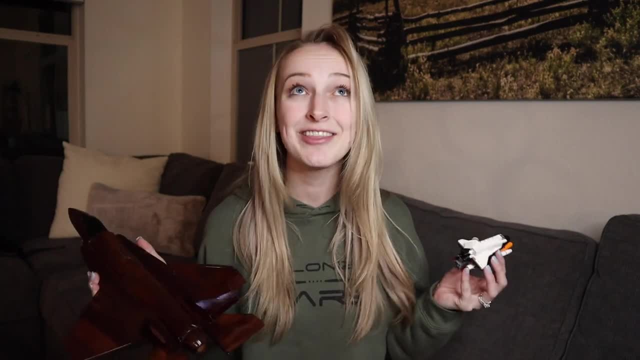 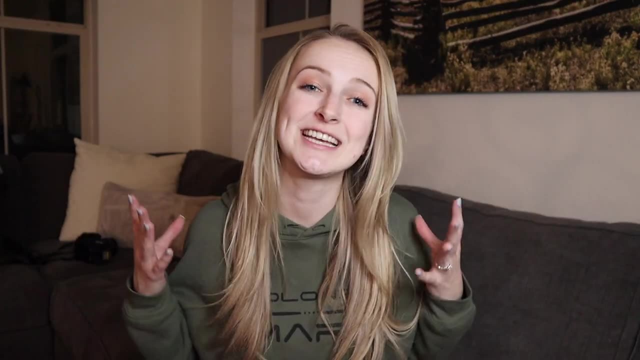 So you literally are air sailing and space sailing, which I think is amazing, because I hate water, so I will never be a water sailor. Throughout this video, we are going to be breaking down aeronautics and astronautics, everything that goes into them, and the types of technologies that you can work on. 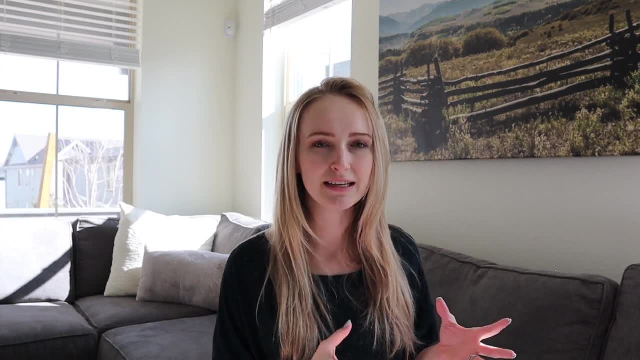 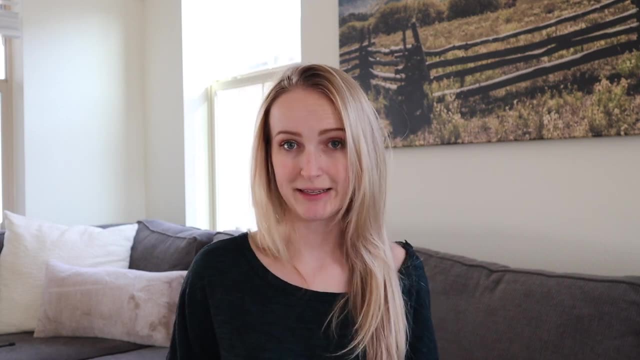 Let's go ahead and start with the aeronautics side of things, The side of things that deals with anything that moves through the air. When people think of the aeronautical side of aerospace engineering, they typically think of planes, But as an aerospace engineer, you can also work on helicopters, drones. 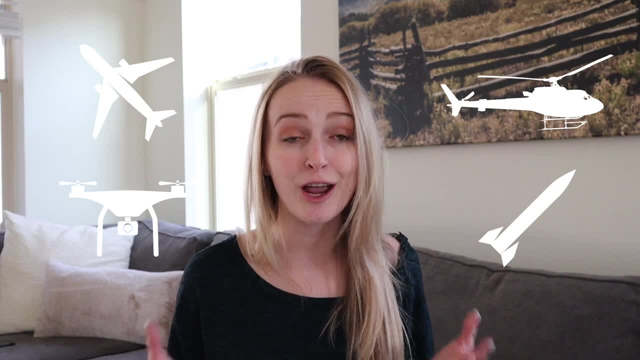 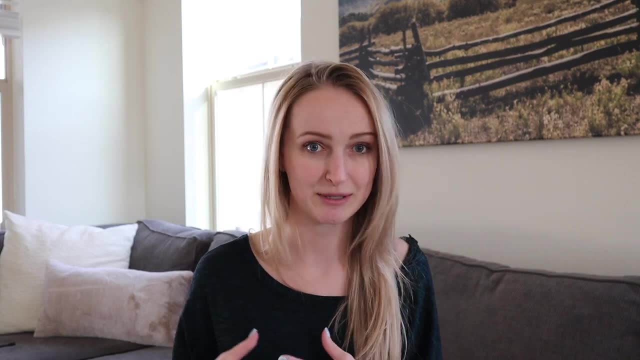 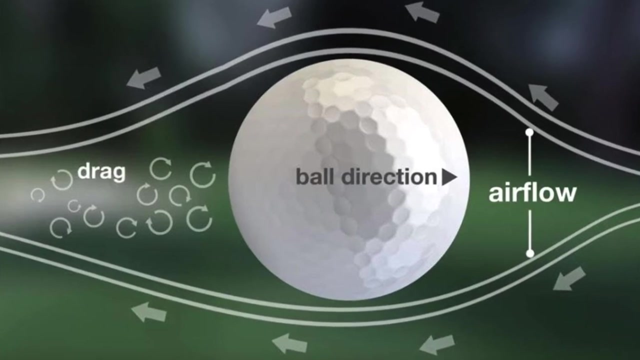 missiles and, honestly, anything that moves through the air, including cars. And another great example of something that isn't a traditional aerospace technology but utilizes the concepts of aerospace engineering are golf balls. So if you look at a golf ball, it has all those dimples right And those dimples help it. 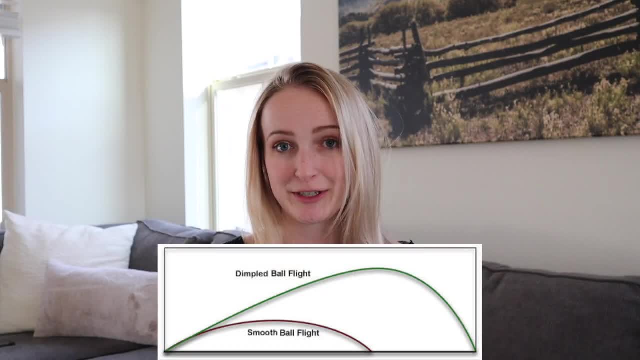 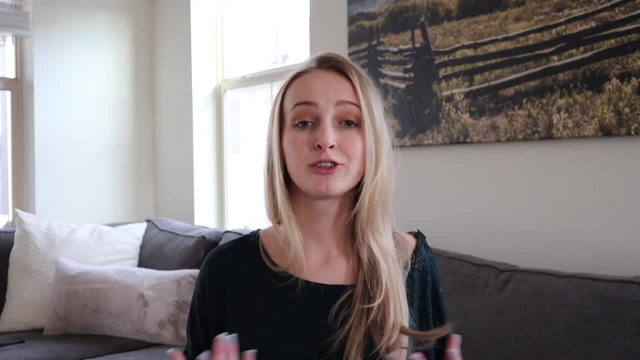 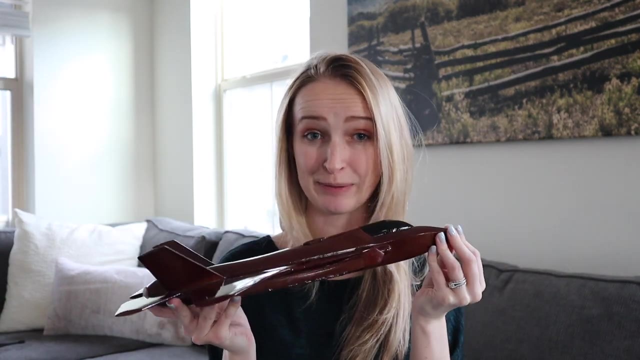 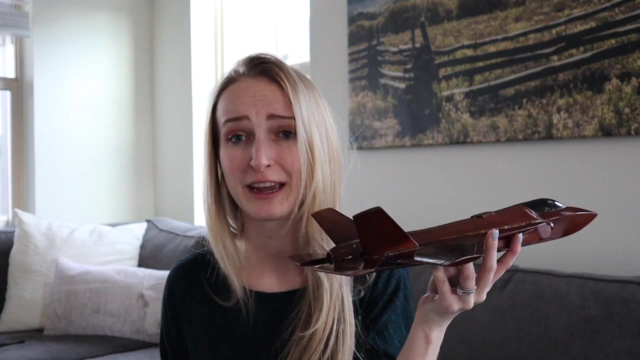 move through the air more efficiently and faster, on a better trajectory, to help golf players with their game. To talk about the concepts involved with aeronautics, we're going to use this plane. There's a lot that goes into designing this piece of technology and, honestly, it blows my mind thinking that this heavier-than-air object can fly through the air at insane speeds that I can't even fathom. 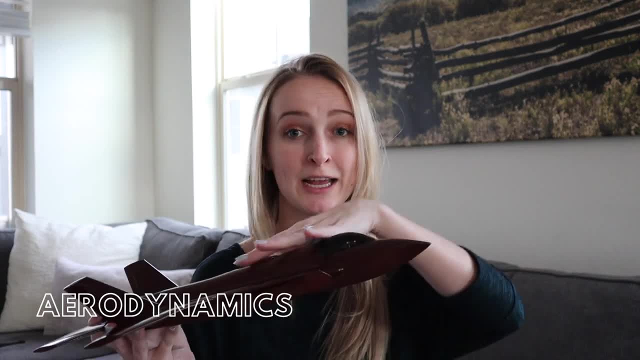 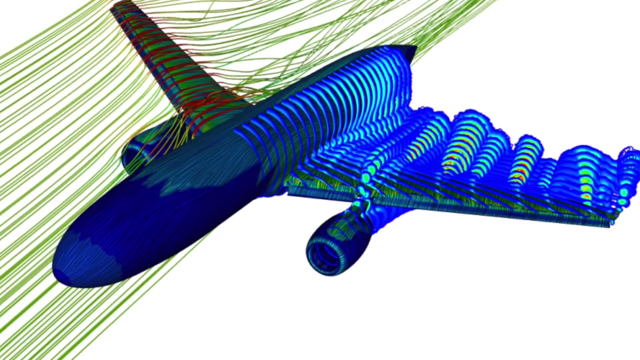 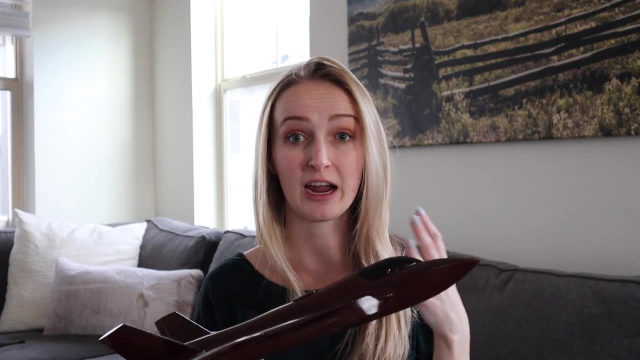 Aerodynamics is the concept of how air and objects interact with each other. as the object flies through the air, As the plane moves through the air, the air flows over each individual part of the airplane, and each individual part has its own shape, its own surface area, its own area that the air actually touches, which affects the overall performance of the airplane. 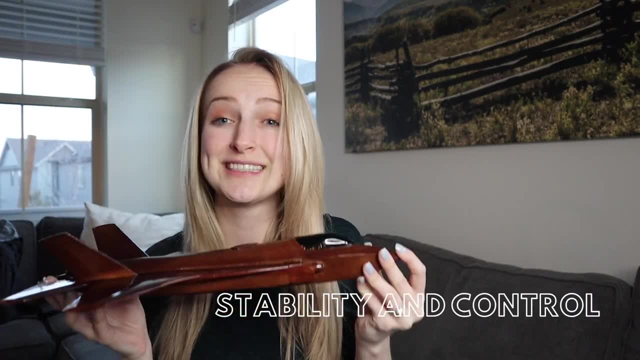 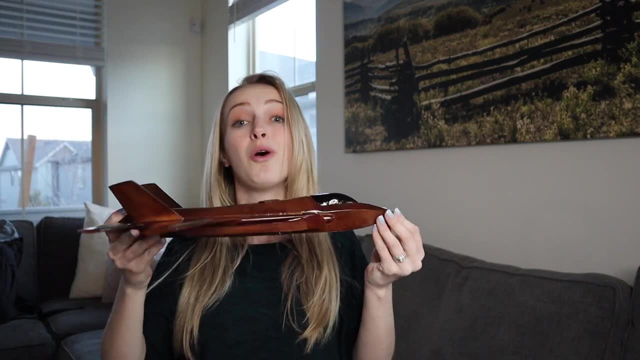 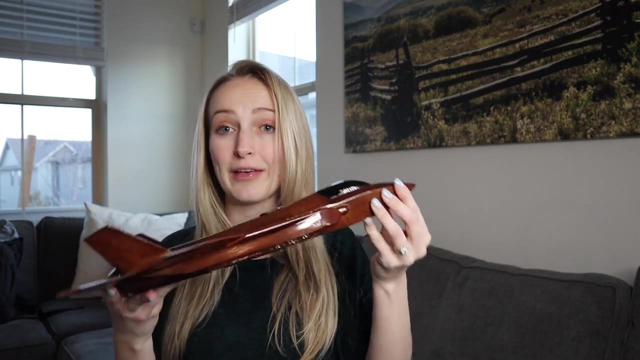 Next up is how you actually control the vehicle while it's in the air. That part of aeronautical engineering is called stability and control, and that is all about controlling the vehicle horizontally and vertically. Stability and control is incredibly important because not only is it how the pilot flies through the air, 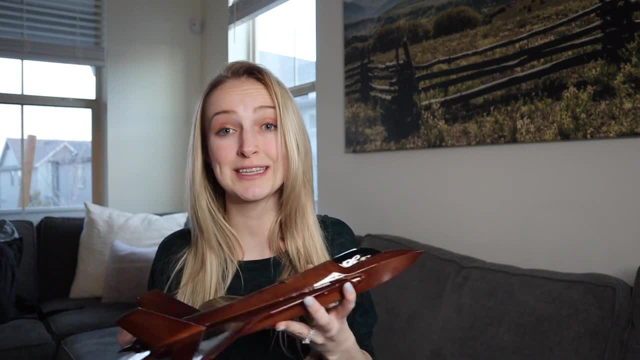 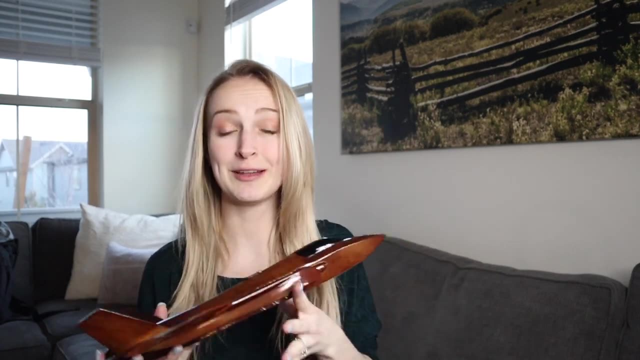 but the plane has to be able to adapt to things like turbulence as it's flying. What the Plan is actually made out of. This is incredibly important because planes and, as we'll see later, spacecraft—they operate in some of the harshest environments. 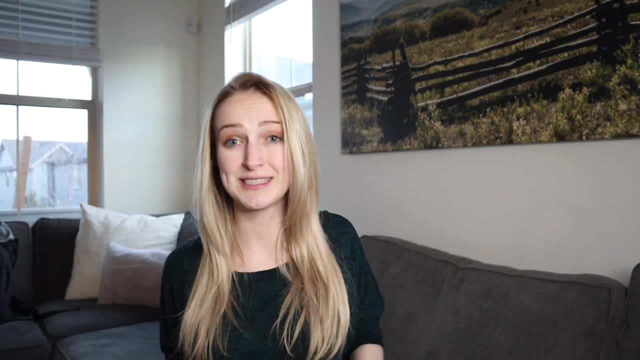 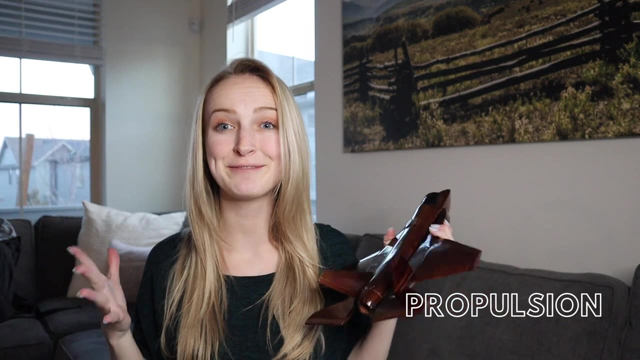 known to mankind, and the materials have a different nature, have to be able to withstand the speed and the heat that the plane is experiencing. So how is the plane powered to move through the air? Well, that is a field called propulsion. Propulsion is a general topic. 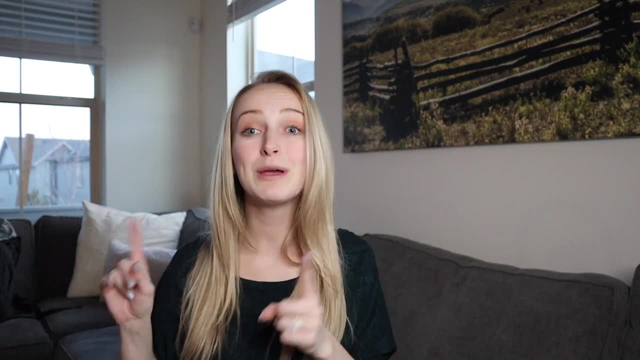 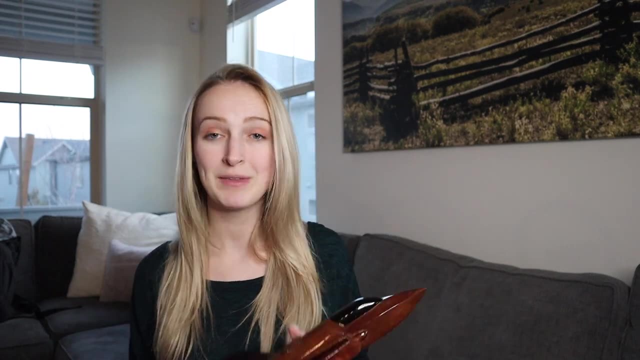 that just means powering these aircraft, spacecraft etc. We will get to rocket propulsion later in this video. but aircraft propulsion- nowadays it is typically a jet engine And here it's kind of hard to see. but you have little air intakes here. 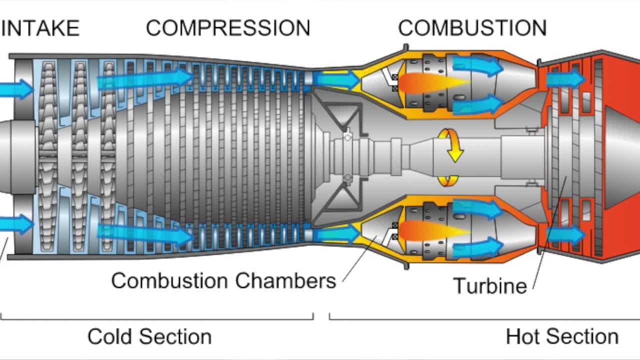 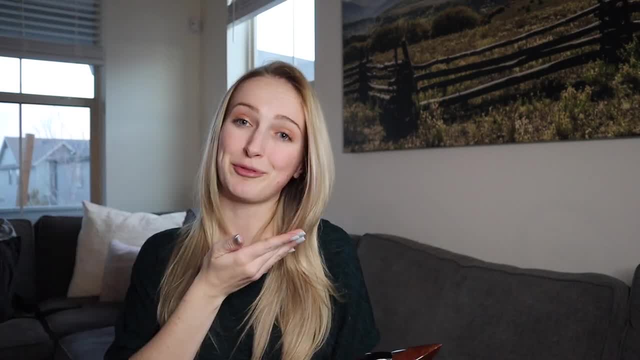 And through a series of steps that is very complicated and too far out of the scope of this video, you get an output of thrust, And thrust is just the force that enables the plane to fly through the air. And the last thing I wanna talk about, 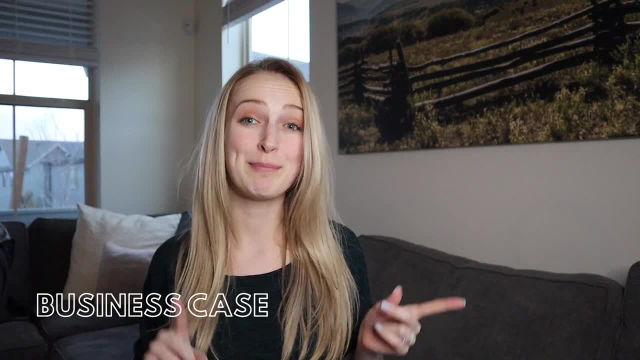 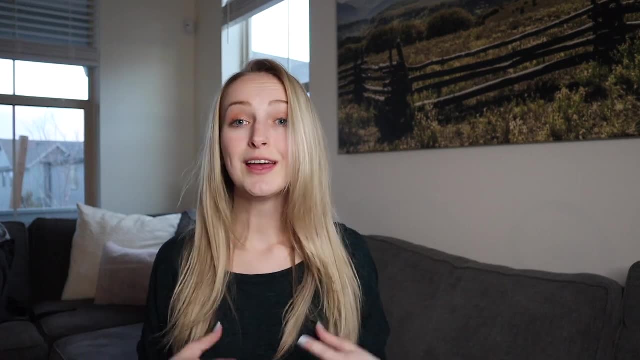 in regards to aeronautical engineering- and you will definitely see this pop up in space as we go forward in this video- but that is the concept of business cases and use cases, So in any type of engineering or, honestly, just in life in general. 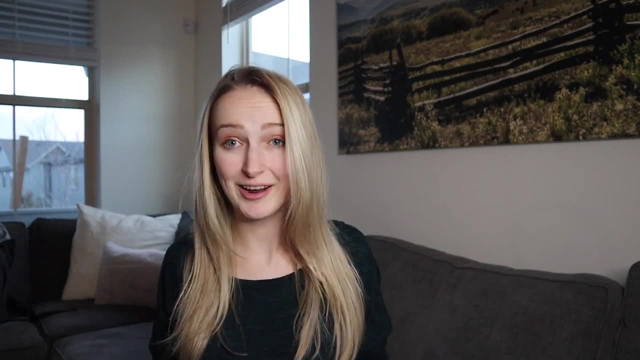 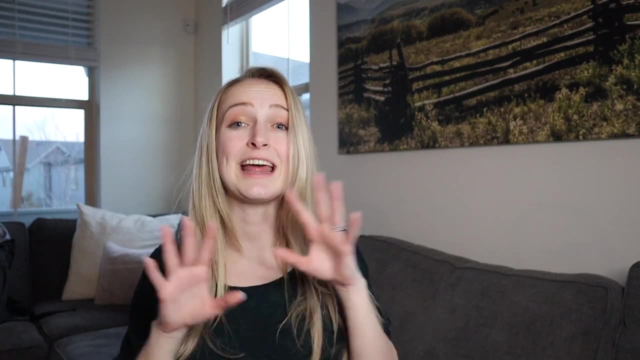 you need a business case for everything And, in regards to aeronautical engineering, you need to understand where your plane is gonna go and what capabilities your plane is going to have, And that will dictate everything else, everything we just talked about: Aerodynamics, stability and control materials. 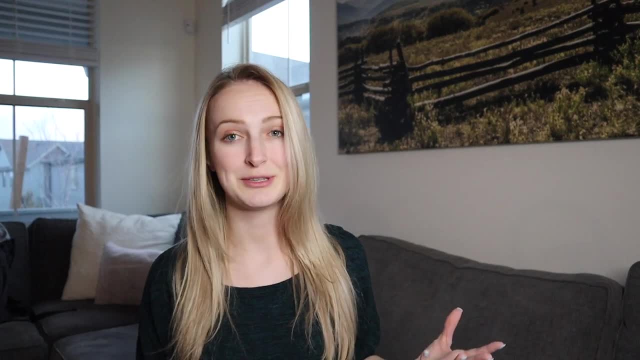 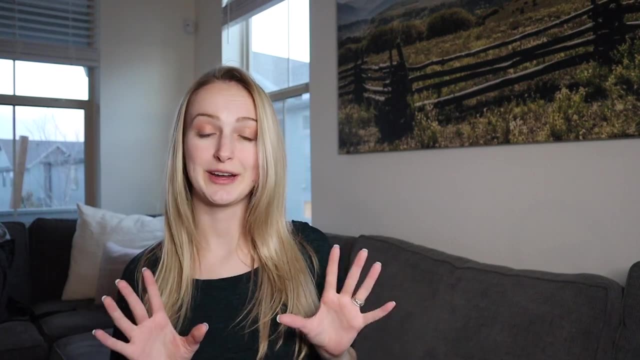 all of the above will be determined by what your plane is going to be used for. So we just went over a bunch of concepts, right? So let's recap. Aerodynamics is the concept of how objects interact with the air as they are flying. 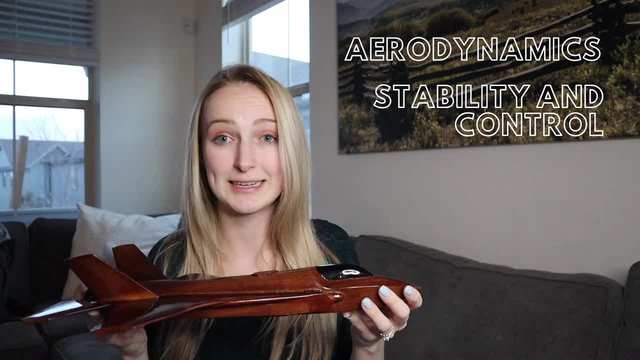 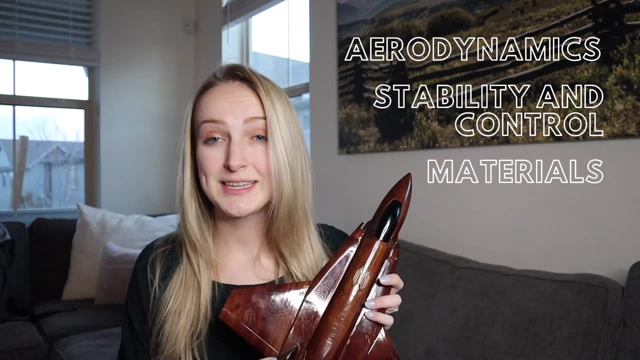 Stability and control is how you control the plane up down, left, right, et cetera- and how it responds to anomalies as it's flying to keep its passengers safe and continue to perform its mission. Material science in the aerospace world is all about. 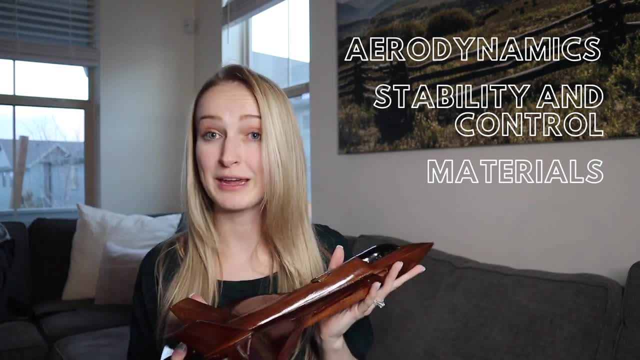 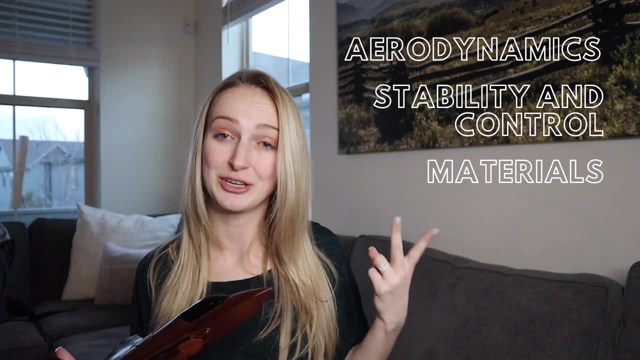 how do you get this plane to go from point A to point B and do its mission without falling apart? basically, What materials do you need to use to operate at the speed and the temperature that you are going? Propulsion is how you power the aircraft. 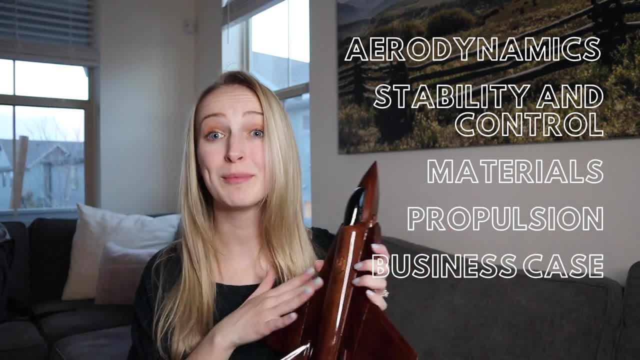 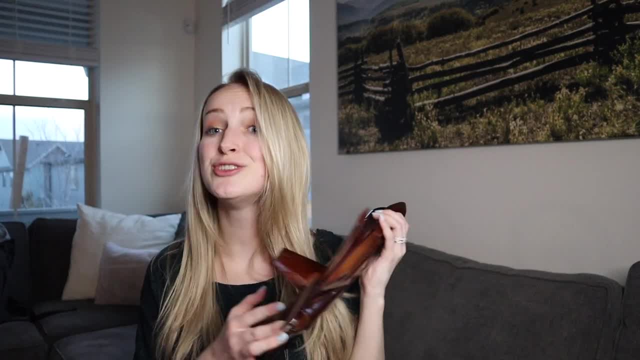 to get it going through the air. And, lastly, your business case determines how you design your airplane. All of these concepts apply to every technology in the field of aeronautics, not just planes, So it applies to helicopters and drones and missiles. 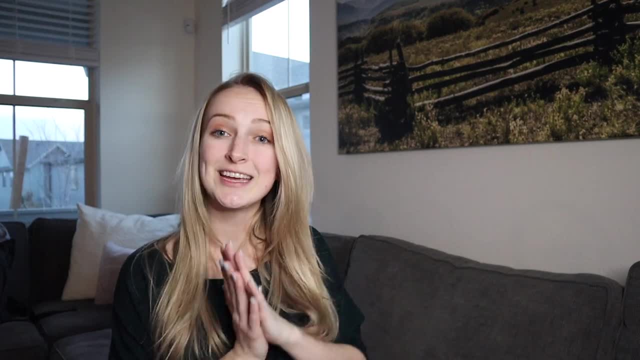 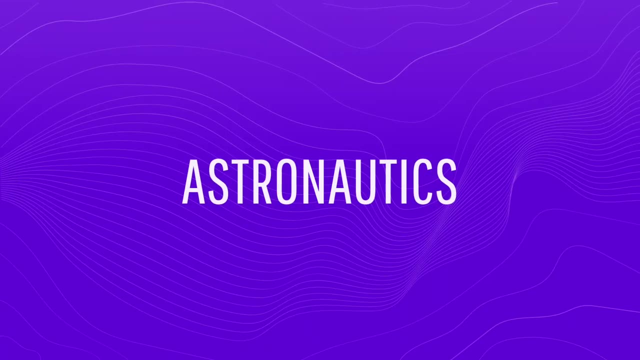 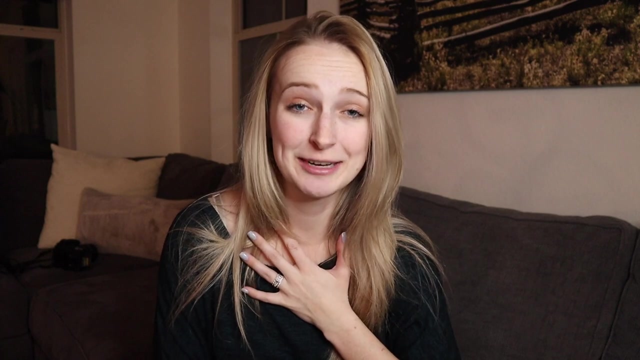 and some of it even applies to things like cars. So that is aeronautics. Let's take a look at astronautics, all things, space, everything that happens outside of our atmosphere. Astronautics encompasses so many different technologies, and I could probably write an entire book on them. 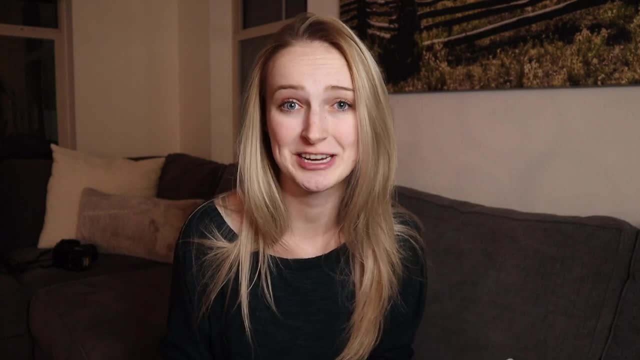 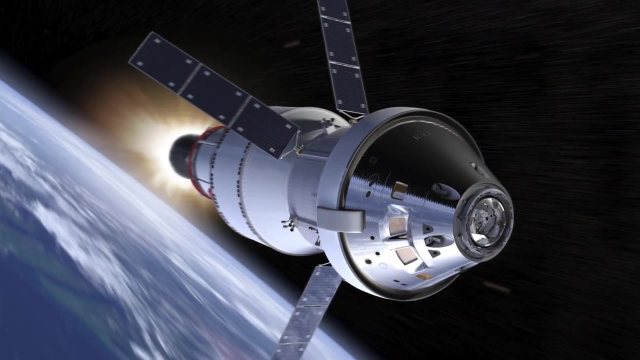 because this is the sector that I work in and I am so, so, so passionate about it. But a few of my favorites are crew capsules like the space shuttle Apollo or Orion that's about to take us back to the moon. Satellites like weather satellites, GPS satellites. 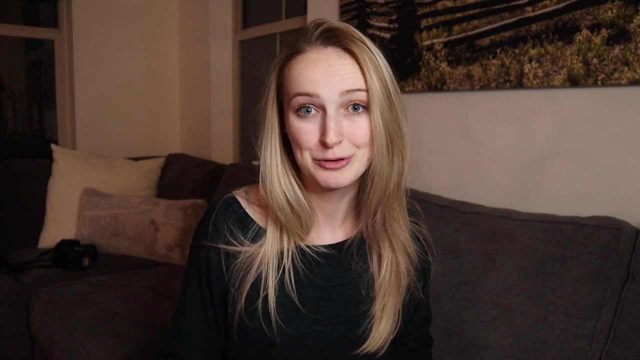 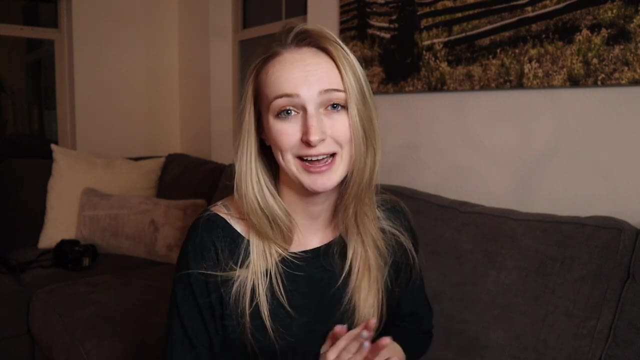 Did you know that when you open your phone and pull up Google Maps, you're actually using a satellite that is beaming you a GPS signal? Life support systems are another really awesome area of astronautics. In fact, there is an entire degree called bioastronautics. 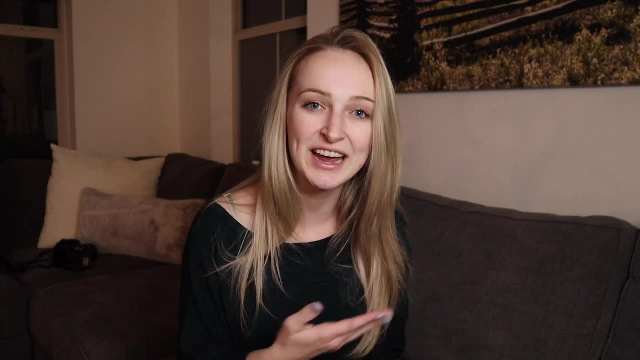 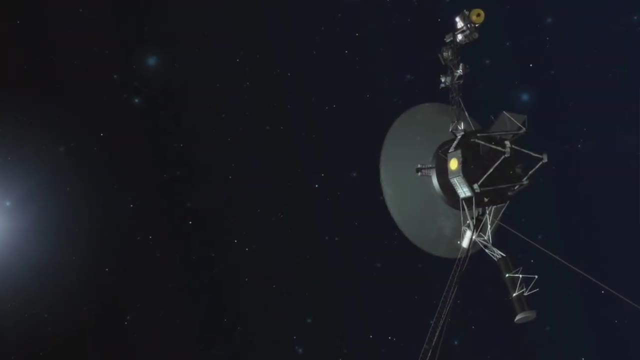 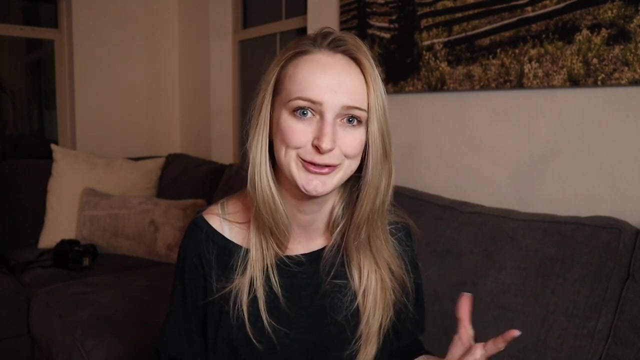 that focuses on how humans live and work in space and the effects of space on our bodies. Okay, what about deep space probes like Voyager or Pioneer, The ones that go super far out into our solar system and study the origins of our solar system and all of our different planets in our solar system? 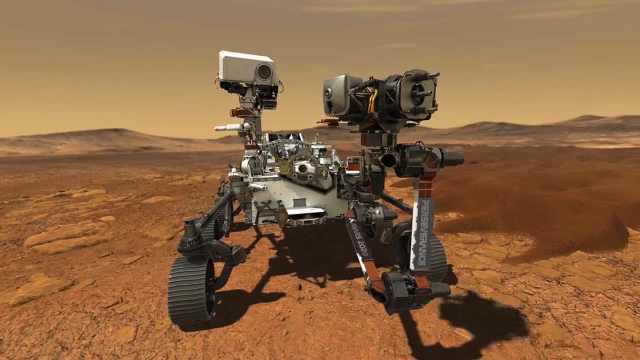 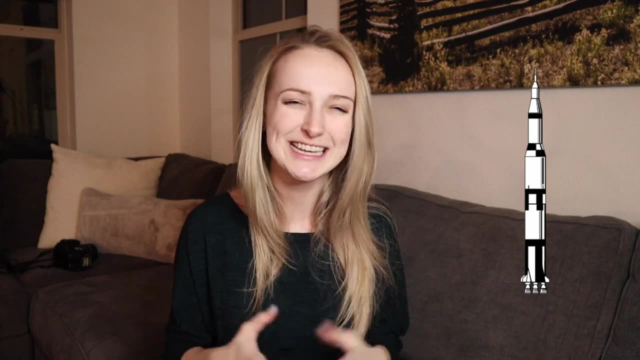 We also have rovers and orbiters and landers that go to the moon and Mars and other planets in our solar system, And then, of course, we could not forget our lovely rockets, The things that actually get us to space In the first place. 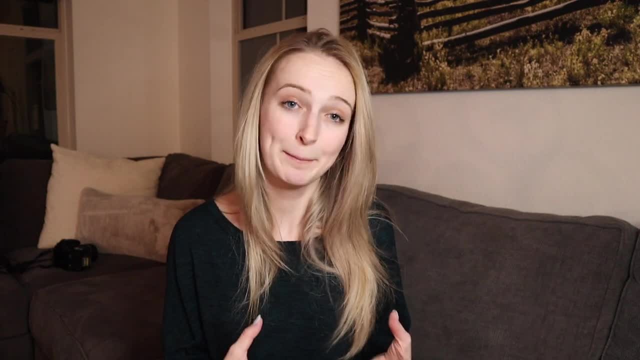 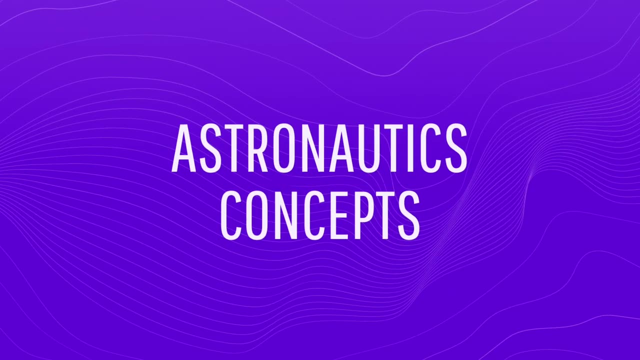 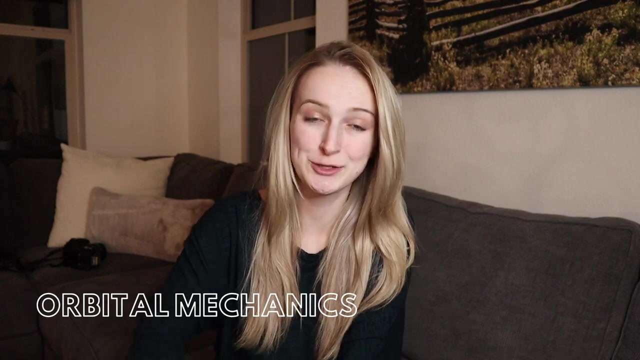 So with all of that, just like we talked about with aeronautics, you have a core set of topics that you would probably be working with if you worked in astronautics in the space industry. So first up, we have orbital mechanics, which is my favorite part of astronautics. 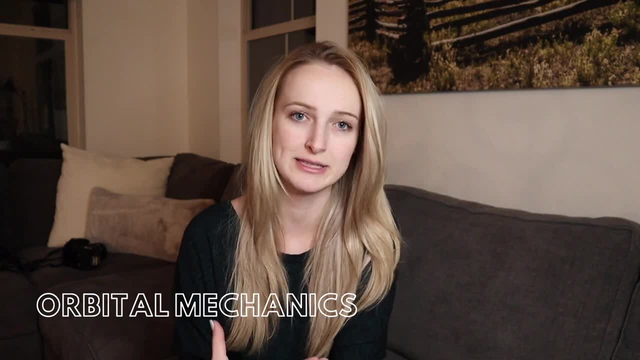 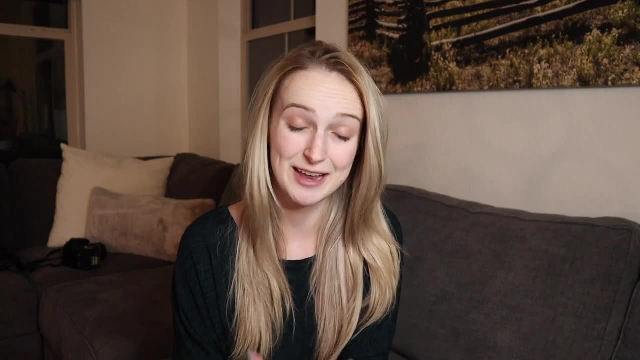 Orbital mechanics is the study of how objects move about in space, how they move about around our earth, around other bodies in our solar system and, ultimately, around our science, and ultimately around our science, because that's what we're very interested in. 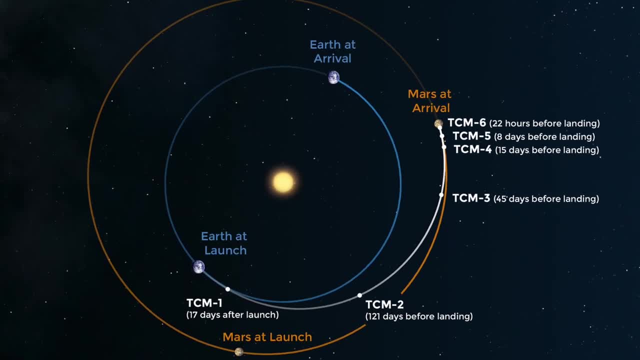 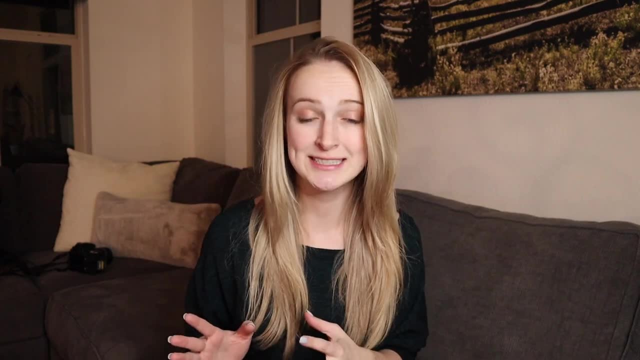 and how we can get that thinking to happen. And it's all done because earth is orbiting the sun. Orbital mechanics also tells you how to get from one place to another in our solar system. Next up we have propulsion. So we talked about propulsion a little bit. 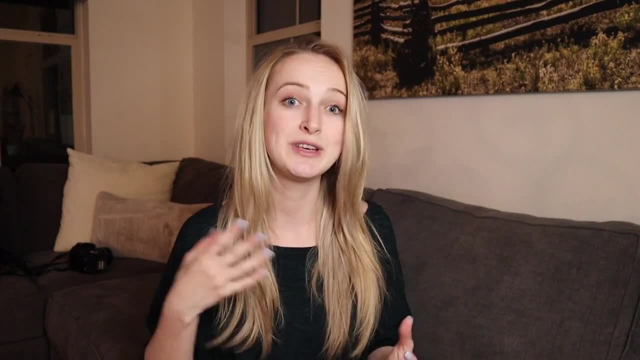 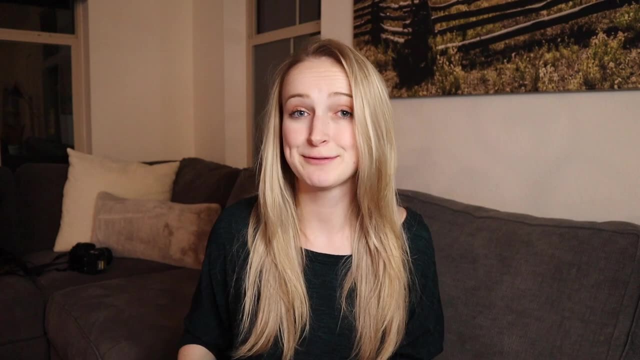 on the aeronautic side of things, On the astronautics side of things, it is the same concept. We are putting energy in to get a thrust out, And a thrust, as we mentioned before, is the force that enables an object to fly. 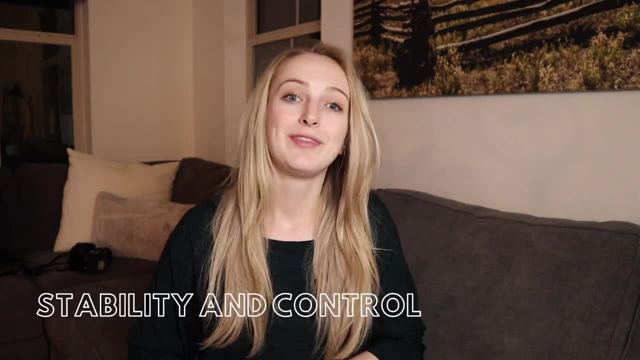 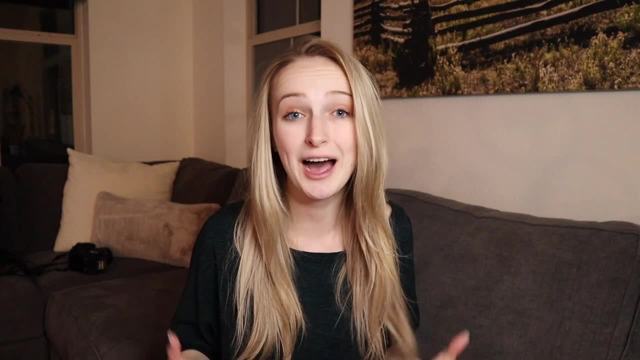 And in the case of a rocket, the thrust is enabling the rocket to fly through the atmosphere. thing we talked about with aeronautics is stability and control. So spacecraft have the same needs that an airplane has. You have to control them, you have to stabilize them, and they have. to be able to maneuver to avoid collisions or to change orbital paths and more Materials are another extremely important part of astronautical engineering, especially on the heat shields. So when you're re-entering an atmosphere, there is a ton of heat and energy that is encompassing your spacecraft and you have to have a material that can withstand those speeds. Material science is also incredibly important when it comes to protecting our astronauts and our electronics from radiation, because we don't have the Earth's atmosphere to block a lot of the radiation that is. 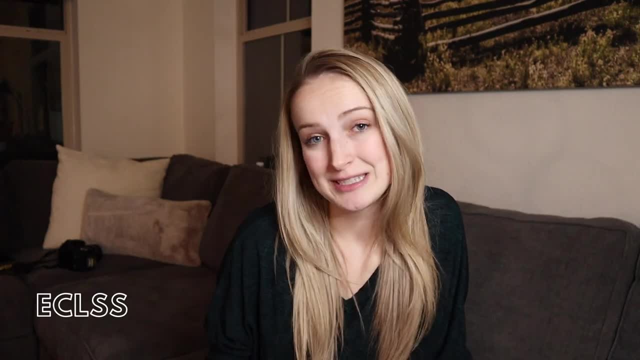 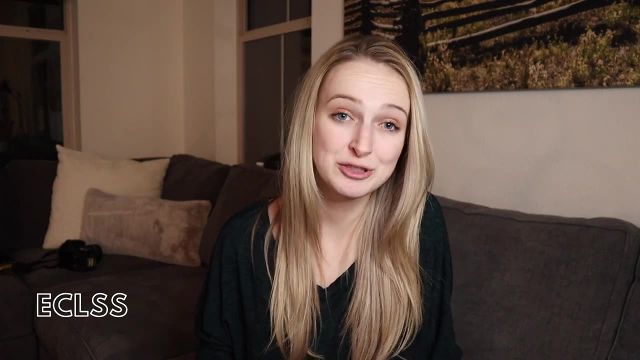 coming from the sun, when we're in outer space, When working with spacecraft that are going to be sending astronauts into space. there's an entire team dedicated to something called ECLSS, which is Environmental Control and Life Support System, and that deals with just making sure that. 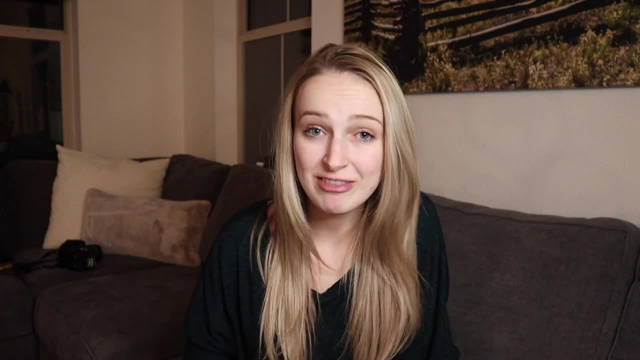 the humans can be able to do what they want to do. So when you're in outer space, you have to be able to communicate with the astronauts, and they can actually live and work in space. So everything that we have down here, that we need to live, they need to have up there, of course, too. 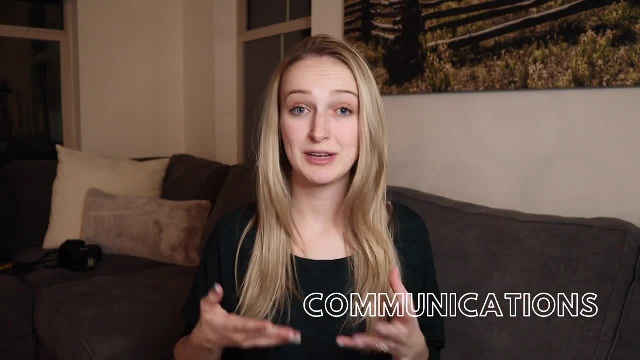 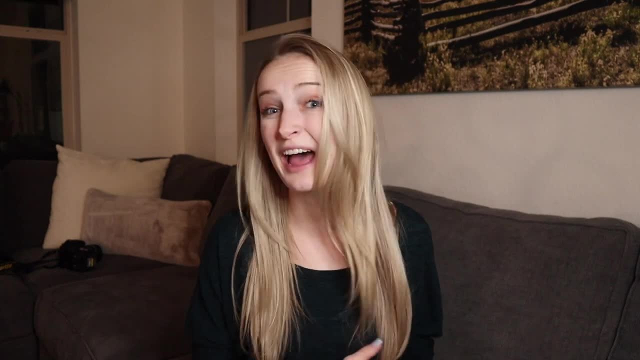 Then we get to communications. So just like we need to be able to communicate with each other down here, the astronauts need to be able to communicate with mission control, but also satellites that don't have any astronauts on them have to communicate with us as well. They have to. 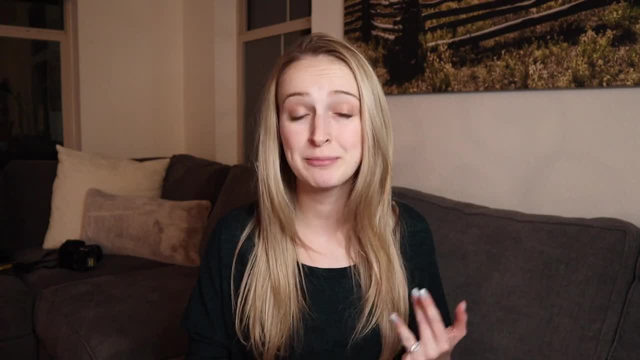 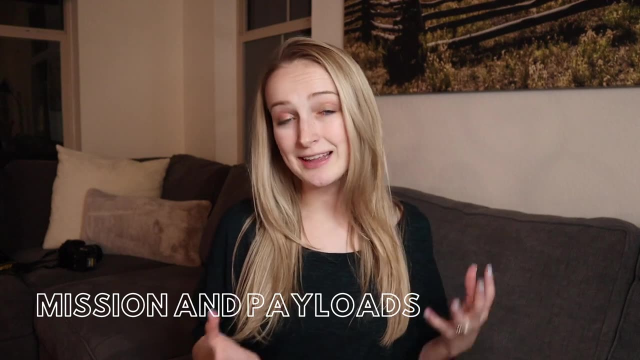 be able to send data down to the ground for their mission, but also just the health and safety of the satellite itself, so that engineers know if they're going to be able to communicate with us. And then, lastly, like we talked about with aeronautics, you need to have a business case. 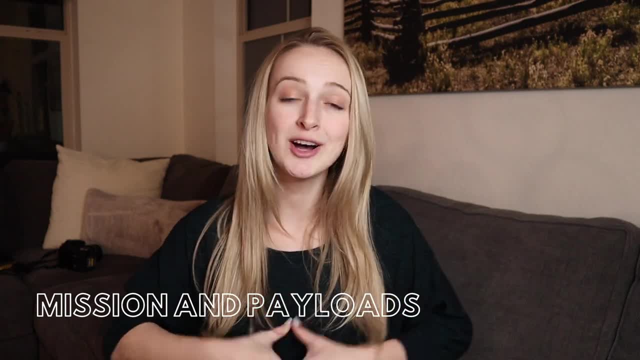 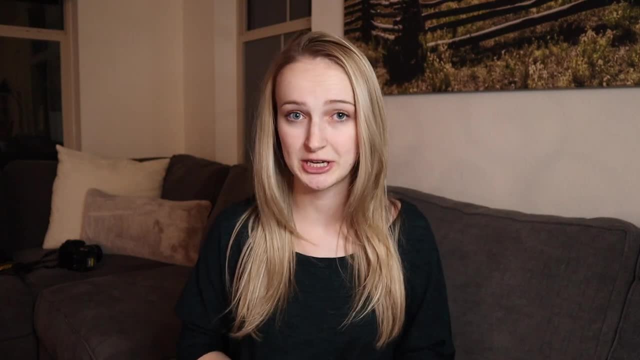 You need to have a purpose, What's your mission? And so on spacecraft, we have what's called payloads. Every satellite has payloads and the payloads just perform the satellite's primary mission. So for a weather satellite, you would have a weather sensing payload. For Mars rovers, 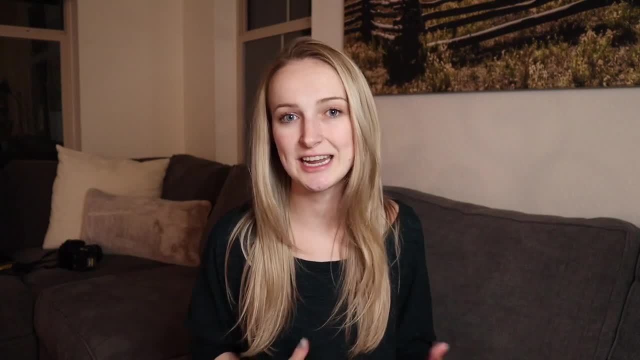 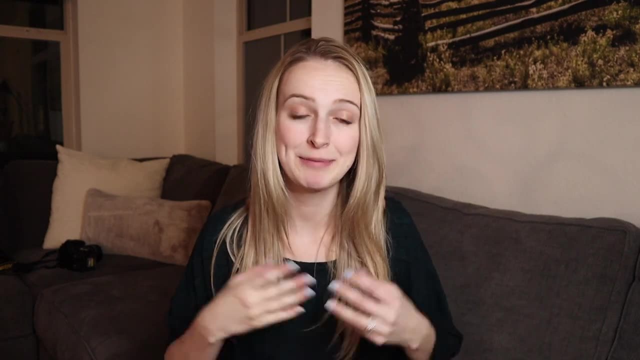 you would have all sorts of scientific payloads that are intended to study different parts of Mars, including the soil, the atmosphere, et cetera. So every spacecraft has a payload and every spacecraft has a mission, And because space and just aerospace in general is very expensive,